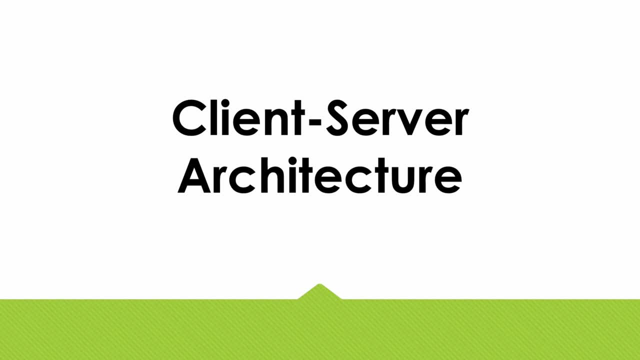 One system acts as the client-initiator and the other system acts as the server hosting the remote desktop service. The client-system runs an RDP client software such as Microsoft Remote Desktop or third-party clients to connect to the remote desktop session hosted by the server. 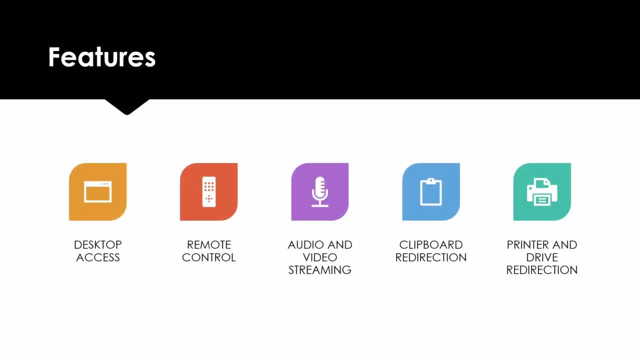 Now we are going to talk about the features of RDP protocol Desktop Access. RDP provides full access to the remote desktop environment, allowing users to interact with applications, files and system links. RDP provides full access to the remote desktop environment, allowing users to interact with applications, files and system links. 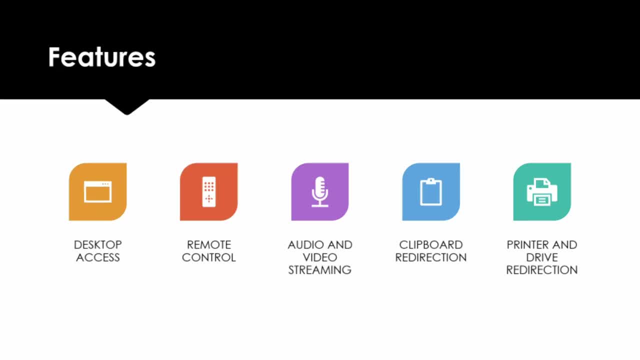 Remote Control. Users can control the mouse and keyboard input on the remote system, enabling them to perform tasks and operations as if they were physically present at the remote location. Audio and Video Streaming. RDP supports audio and video streaming, allowing users to listen to audio and watch videos from the remote system during the remote session. 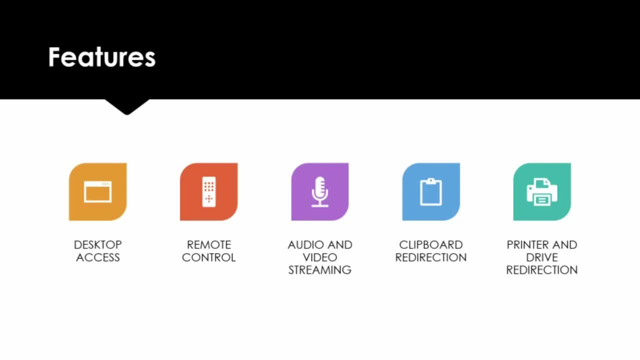 supports clipboard redirection, enabling users to copy and paste text and files between the local and remote system seamlessly. printer and drive redirection RDP allows local printers and drives to be redirected to the remote session, enabling users to print documents. printer and drive redirection RDP allows local printers and drives to be redirected to the remote session. 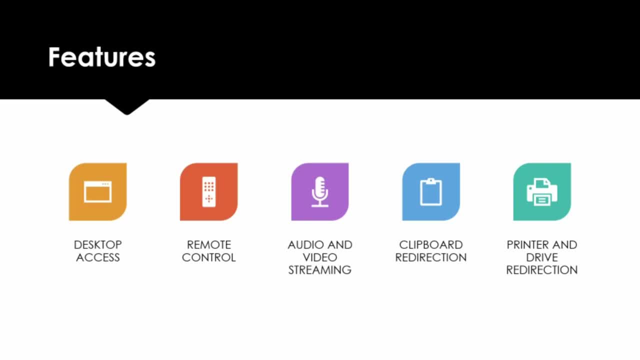 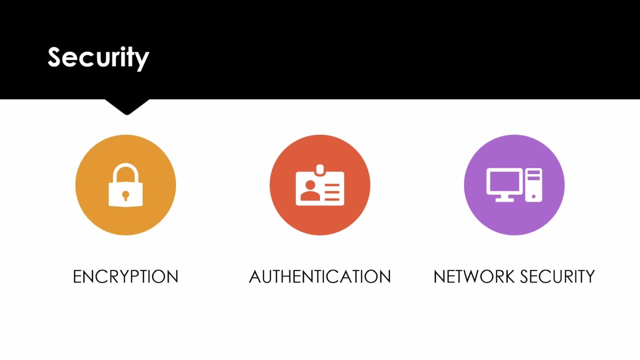 enabling users to print documents and access files stored on their local devices. Security in RDP protocol Encryption: RDP encrypts data transmitted between the client and the server using encryption algorithms to ensure the confidentiality and integrity of the remote session. Authentication: RDP supports various authentication mechanisms, including password-based authentication. 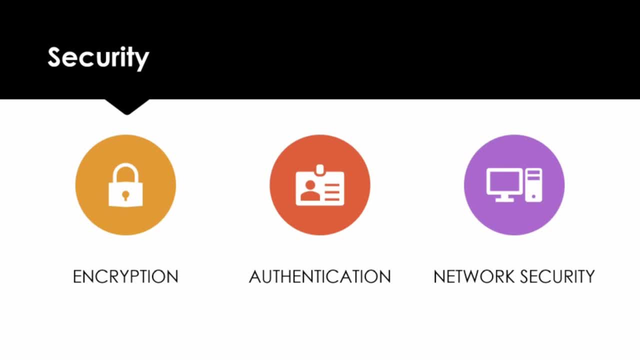 network access authentication, or NLA, and multi-factor authentication MFA to verify identity of users connecting to the remote session. Network security RDP can be configured to operate over secure network protocol such as TLS, SSL, to protect against eavesdropping and man-in-the-middle attacks. 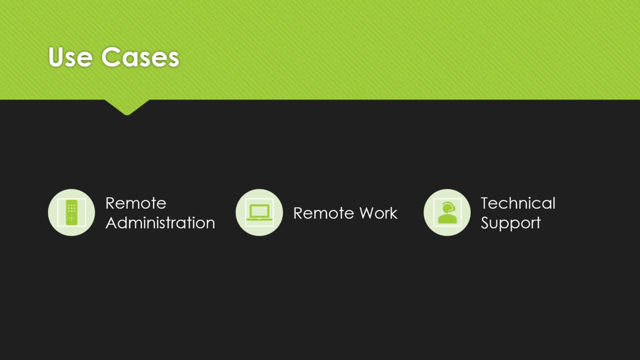 Use cases. Remote administration- RDP is commonly used by system administrators to remotely manage servers and desktop systems, perform maintenance tasks and troubleshoot issues without the need for physical access to the remote systems. Remote work RDP enables employees to access their work desktops and applications remotely. 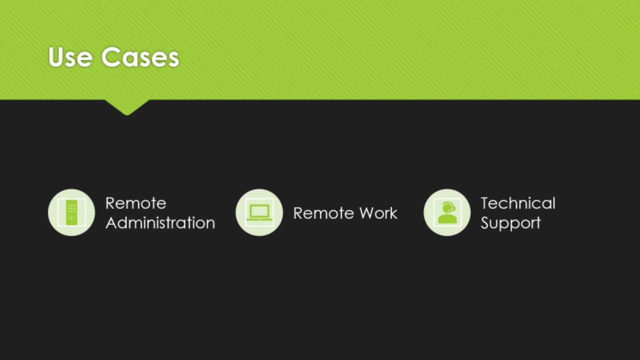 facilitating remote work and telecommuting arrangements. Technical support- RDP allows IT support personnel to remotely assist users with troubleshooting issues, installing softwares and resolving technical problems. Now we will see how to remotely access a computer with the RDP protocol. Enter the hostname of the remote system you'd like to access and press connect. 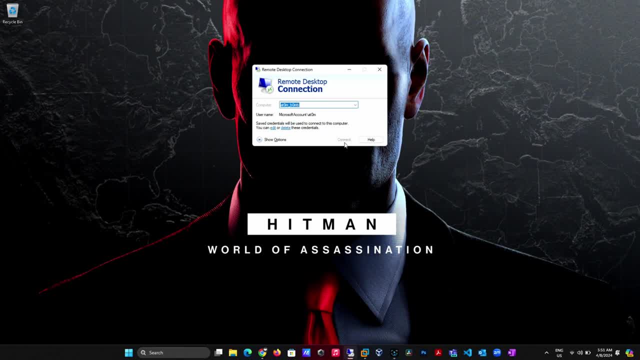 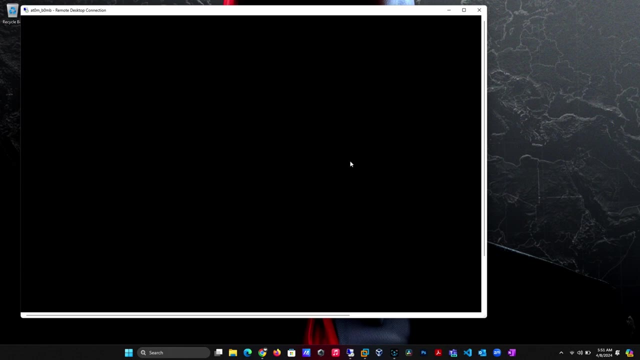 The system will not ask for user credentials as I've saved them in the form. You can see that I'm going to get a certificate error that if the ID of the computer is not verified, I just have to click on yes. When difficult to use a computer to love RDP, the system can be easily strangled into the copy and paste it. 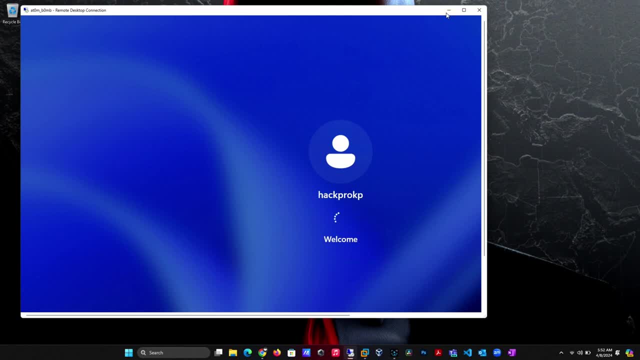 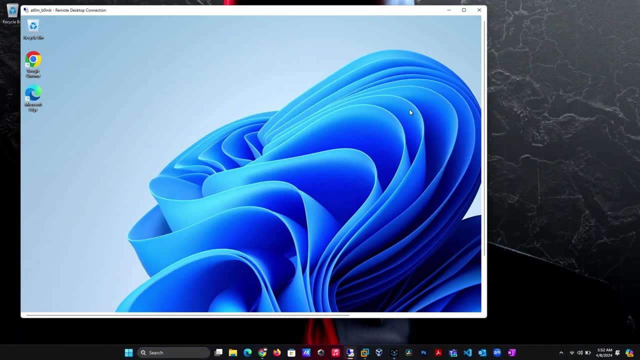 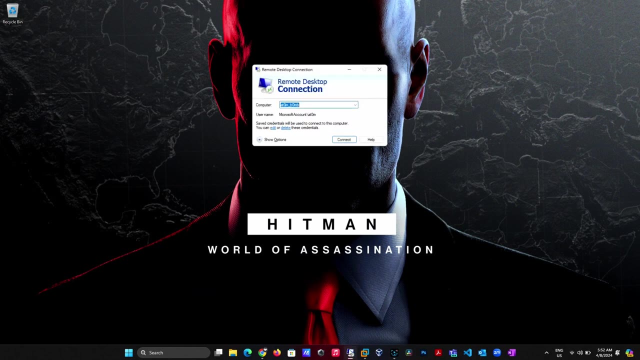 Now the server can enjoy the system on file and save it that i am able to access the remote server by using the remote desktop connection application. now we will see how to access a remote server by mentioning the ip address in the computer field. just write the ip address of the remote system and press the connect button. 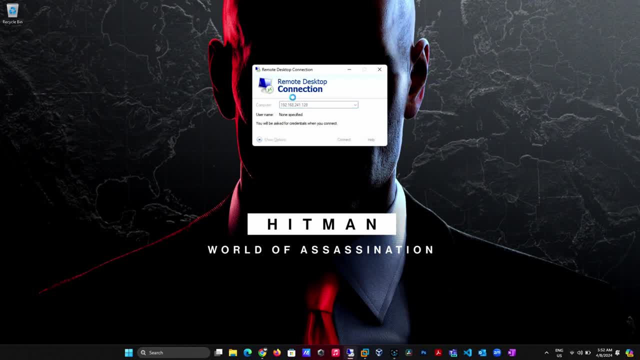 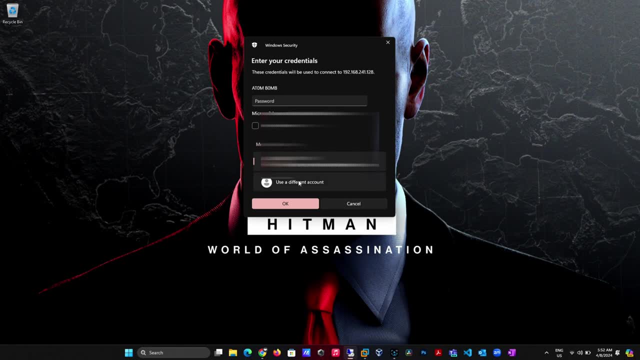 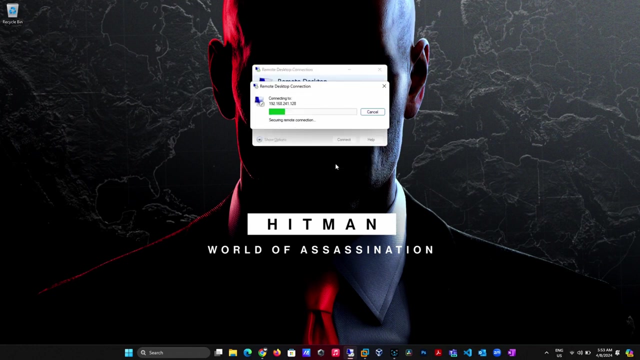 you can see that it is asking for my user credentials to access the computer. i am going to quickly enter those details and press on the ok button. you can see that i got the same invalid certificate error. you just have to click on yes and continue. now we will see how to access the remote server by mentioning the ip address in the computer field. 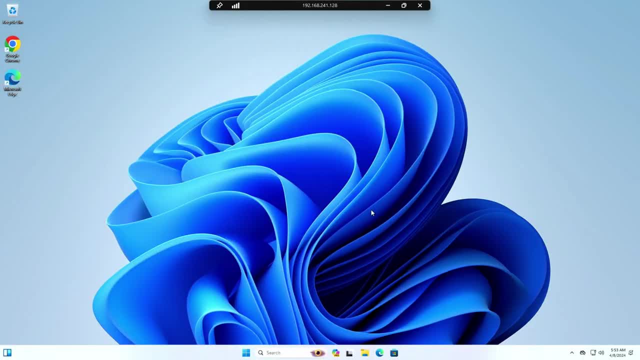 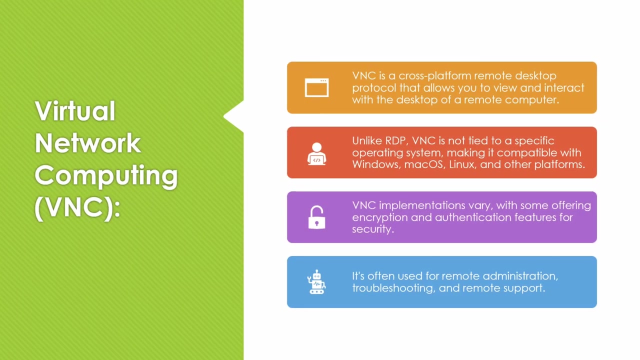 and that's how you can rdp into a remote server and access all the files, open applications and copy paste files and documents between your local and the server computer. now let us talk about virtual network computing, or vnc. vnc is a remote desktop protocol that allows users to view and 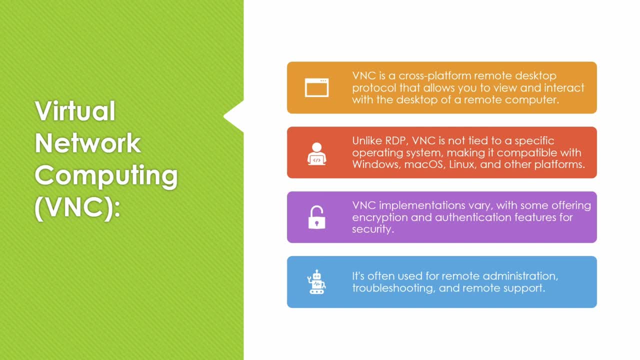 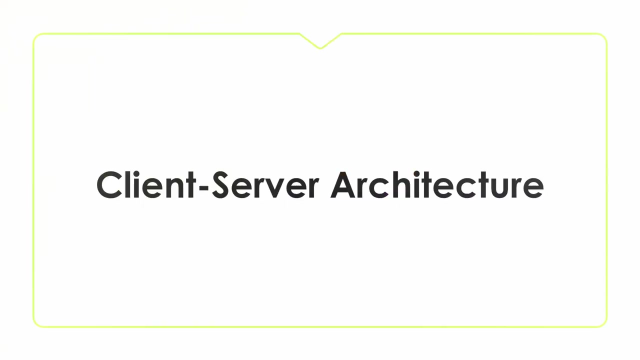 interact with the desktop interface of the remote computer over a network connection. unlike other remote access protocols like rdb, remote desktop protocol, vnc is platform independent, meaning it can be used to access desktop environments on various operating systems, including windows, mac os, linux and others. here's a detailed overview of vnc client server architecture. 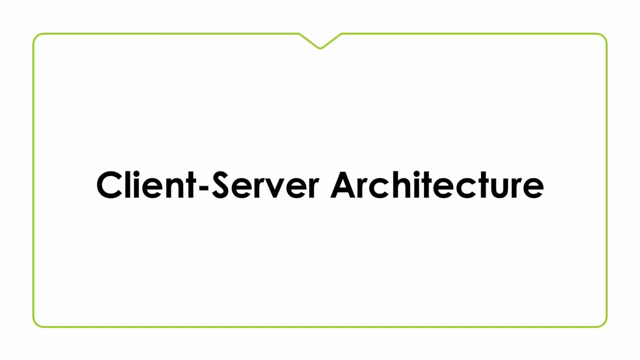 vnc operates on a client server architecture model similar to rdb. the vnc server software runs on the system hosting the desktop session that the user wants to access remotely. the vnc client software runs on the local system allowing the users to connect to the remote desktop session. 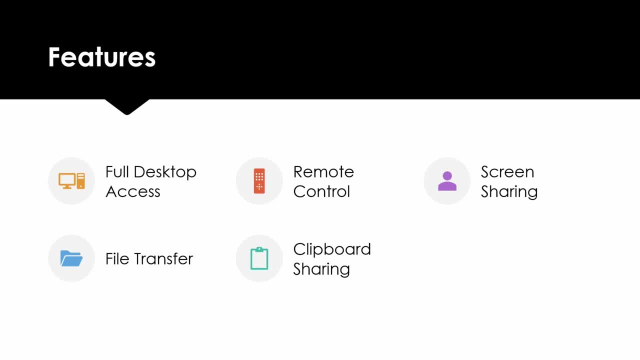 features: full desktop access. vnc provides users with full access to the remote desktop environment, allowing them to interact with applications, files and system resources on the remote system. remote control users can control the mouse and keyboard input of the remote system, enabling them to perform tasks and operations. 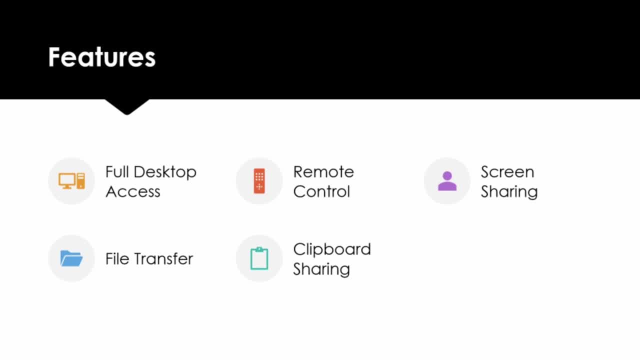 as if they were physically present at the remote location. screen sharing- vnc supports screen sharing allowing multiple users to connect to the same desktop session simultaneously and collaborate in real time. some vnc implementations include file transfer capabilities, allowing users to transfer files between the local and remote system during the remote session. 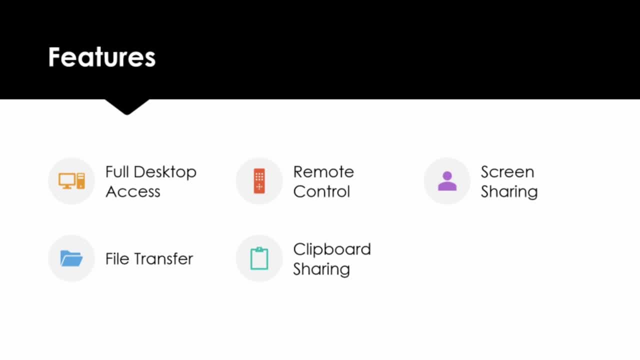 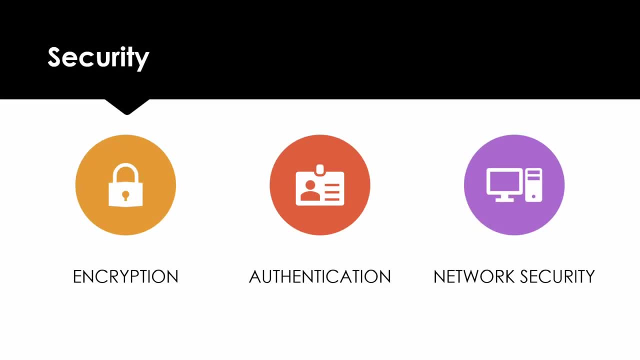 clipboard sharing vnc supports clipboard sharing enabling users to copy and paste text and files between the local and remote system seamlessly. security encryption: many modern vnc implementations support encryption to secure data transmitted between the client and the server over the network. encryption helps secure the confidentiality and integrity of the remote session. authentication vnc. 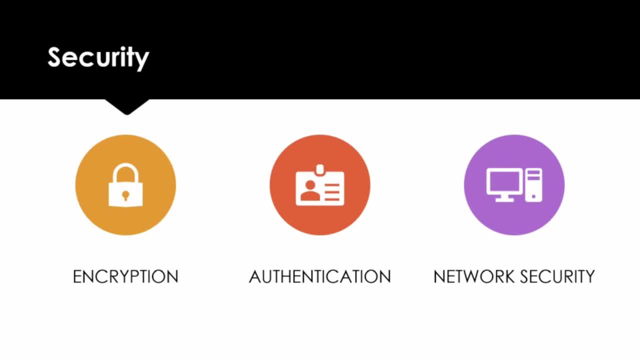 support authentication mechanism to verify the identity of users connecting to the remote session. this may include password based authentication, such as username password authentication or other authentication methods. network security: vnc sessions can be tunneled through secure network protocol such as ssh- that is, secure shell- or vpn virtual private network, to enhance security and protect against. 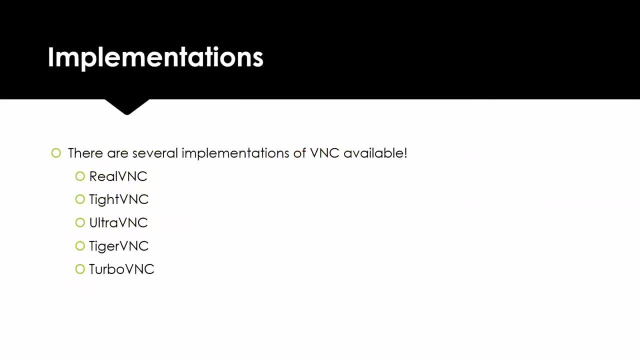 eavesdropping and unauthorized access Implementations. There are several implementations of VNC available, both open source and commercial, each with its own features and capabilities. Some popular VNC implementations include RealVNC, TightVNC, UltraVNC, TigerVNC. 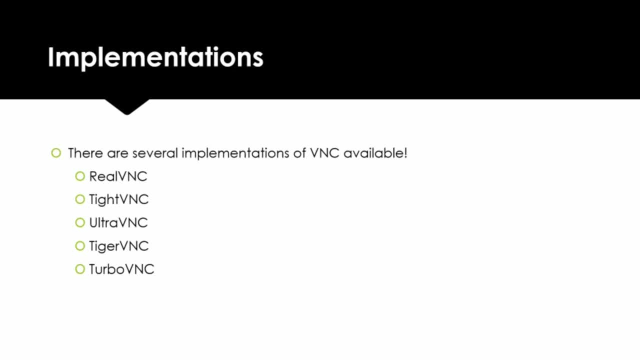 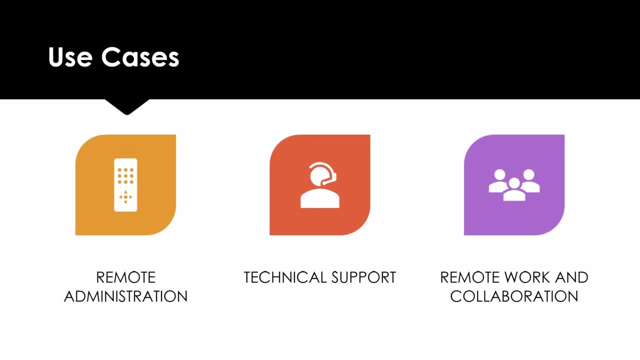 and TurboVNC. Each implementation may offer additional features or optimization tailored to specific use cases, such as performance improvement, platform compatibility or enterprise-grade security features. Use Cases: Remote Administration: VNC is commonly used by system administrators to remotely manage servers, desktop systems and virtual machines perform. 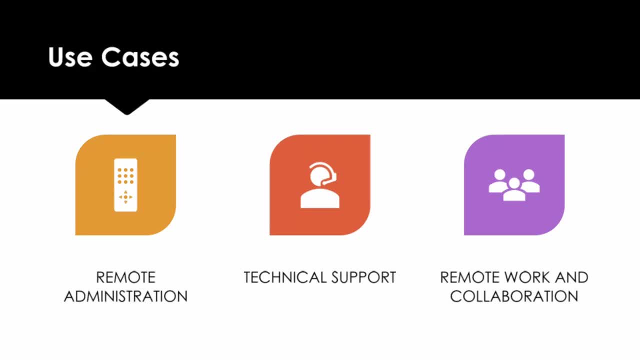 maintenance tasks and troubleshoot issues without physical access to the remote systems. Technical Support VNC allows IT support personnel to remotely assist users and troubleshoot issues like installing softwares and resolving technical problems on their computer. Remote Work and Collaboration VNC enables remote workers to access the work. 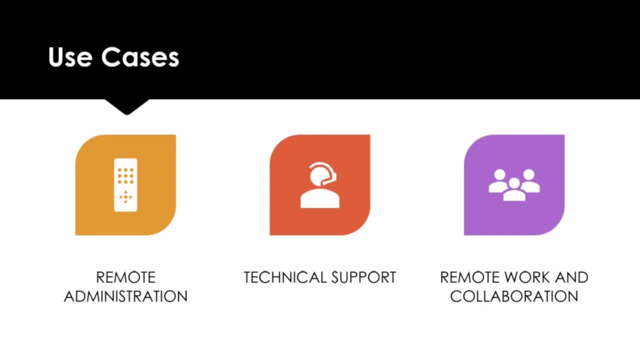 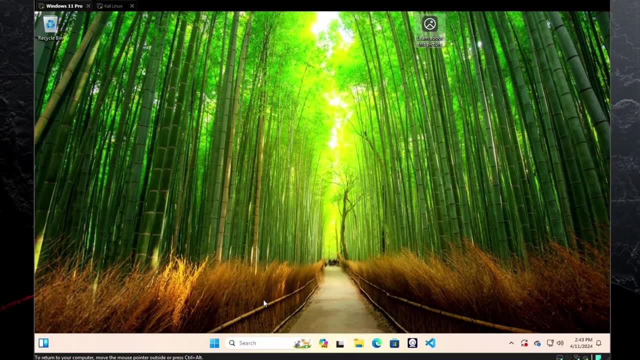 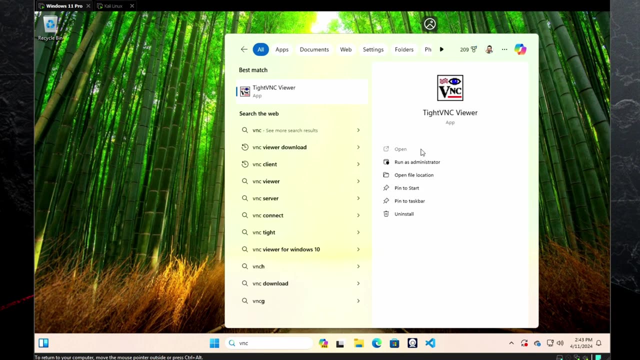 desktop and collaborate with colleagues in real time, felicitating remote work agreements and remote team collaborations. Now we will see how to remotely access a system by using VNC protocol implementations. I am using TightVNC client to access a KarelNex. 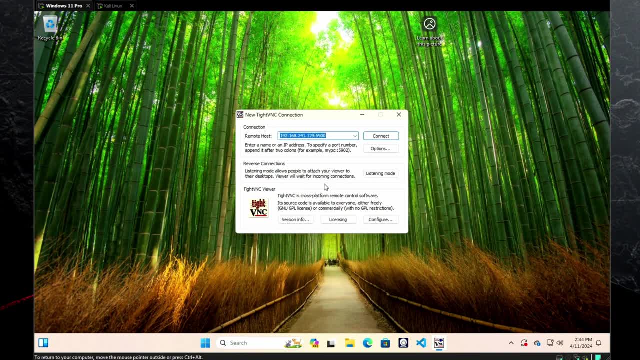 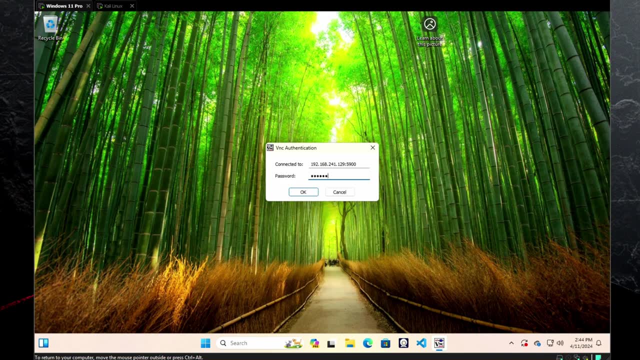 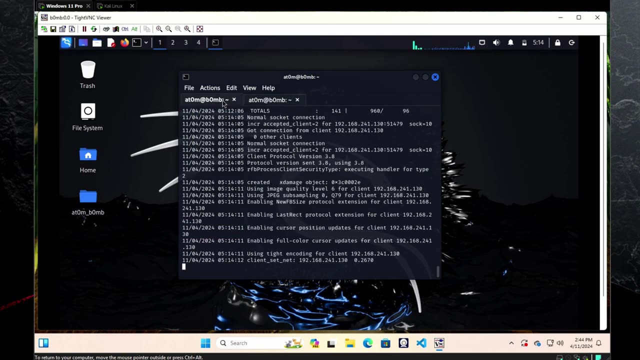 server. I just need to enter the IP address, colon port on which the service is running. The server is asking me to authenticate by using a password. You can see that I am able to access the KarelNex server by using my Windows virtual machine. You can see that. 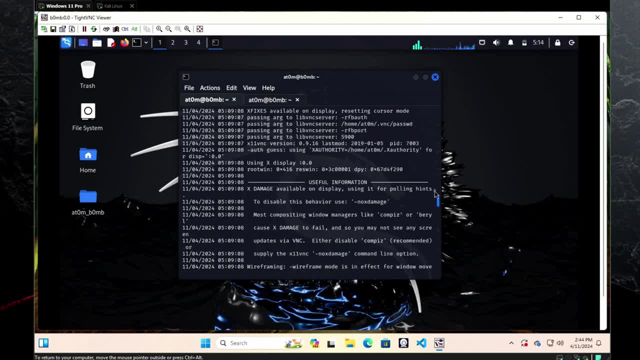 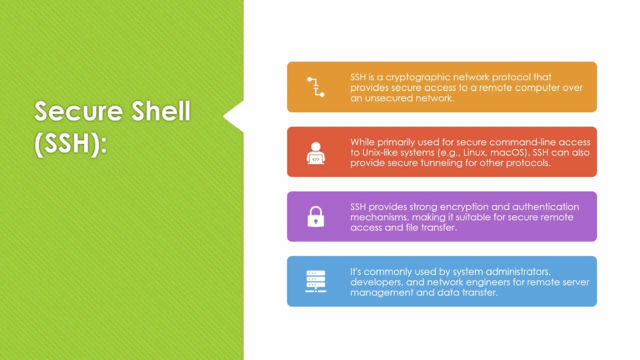 the logs that were generated when I connected to this machine And you can also see I have configured VNC on the server. Now we are going to talk about Secure Shell or SSH. It is a cryptographic network protocol that provides secure communication over an unsecured network. SSH is commonly used for remote access of Unix-like operating systems. 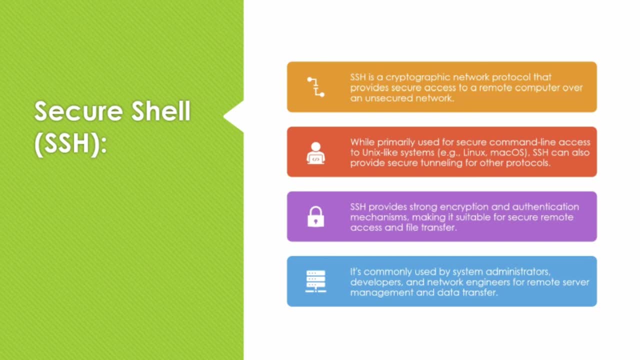 but can also be used for secure communication and data transfer between network devices. Here is a detailed overview of SSH Encryption and Authentication. SSH encrypts data transmitted by the network to a network device. This is called a cryptographic network protocol or SSH. It is a cryptographic network protocol that provides secure communication. 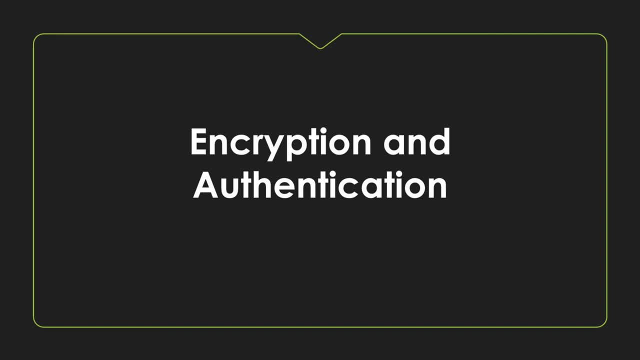 over an unsecured network between the client and the server. to ensure confidentiality and integrity, It uses cryptographic algorithms to protect against eavesdropping, tampering and other security threats. SSH supports various authentication methods to verify the identity of users connecting to the remote system. Common authentication methods include password-based. 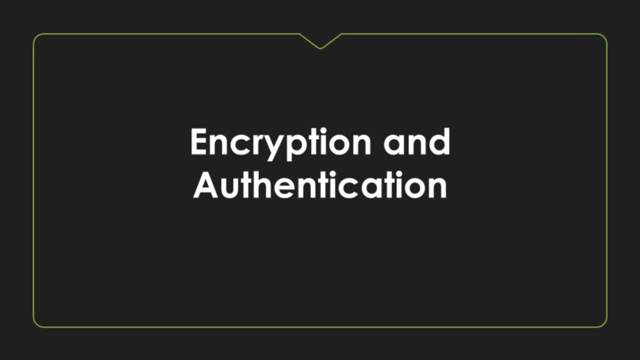 authentication: public key authentication and host-based authentication. Public key authentication is often preferred for its security and security. It is also a good way to identify the server or the network. to ensure the identity of the user. benefits allowing users to authenticate without transmitting passwords over the. 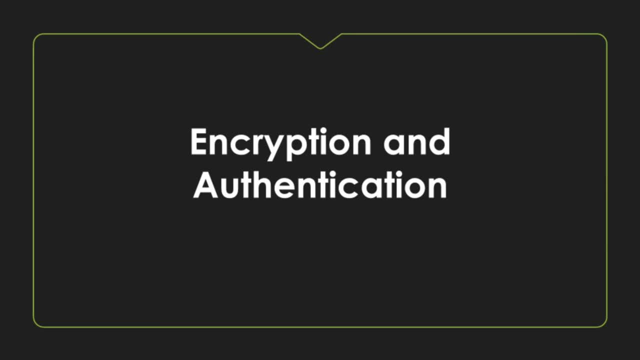 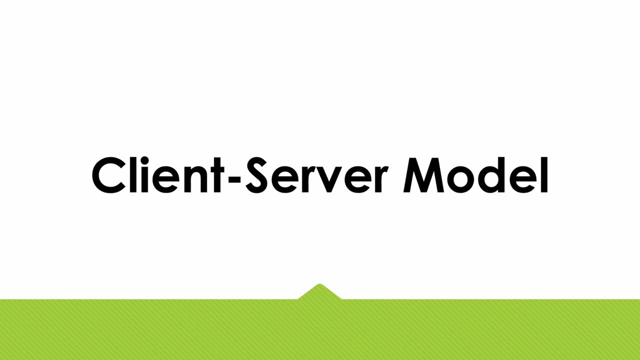 network. it involves the exchange of cryptographic key pairs, where the client possesses a private key and the server holds the corresponding public key. client-server model. SSH operates on a client-server model. we have one system. the SSH clients initiates a connection to another system, the SSH server, to 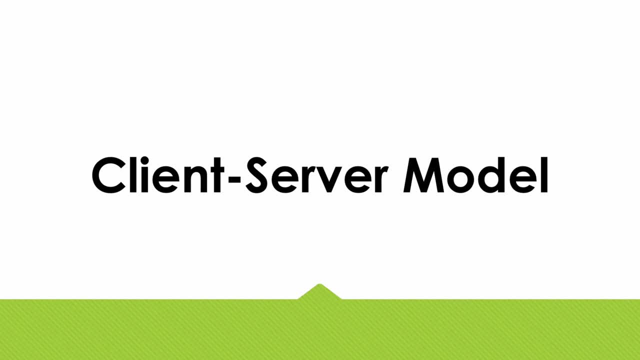 establish a secure communication channel. the SSH client software is typically installed on the users local system, allowing them to connect to the remote system and access their command line interface or execute commands remotely. the SSH server software runs on the remote system, listening for incoming SSH connections and authenticating users attempting to connect to it. terminal. 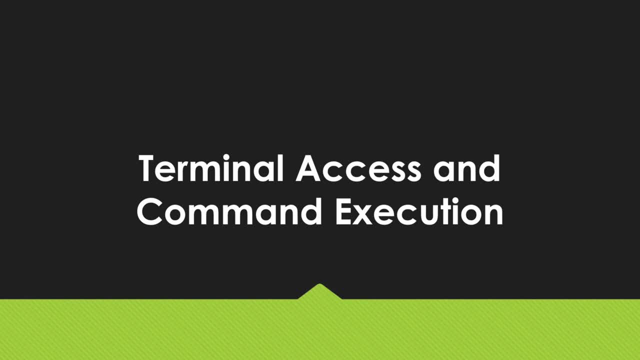 access and command execution. SSH provides users with secure command line access to a remote system, allowing them to execute commands, run scripts and perform administrative task remotely. users can open a secure ssh session to a remote system and interact with its command line interface as if they were physically present at the 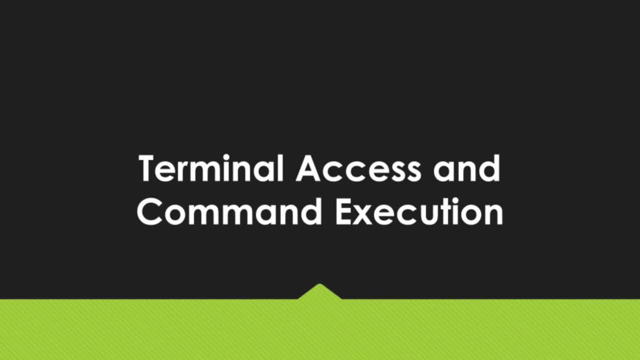 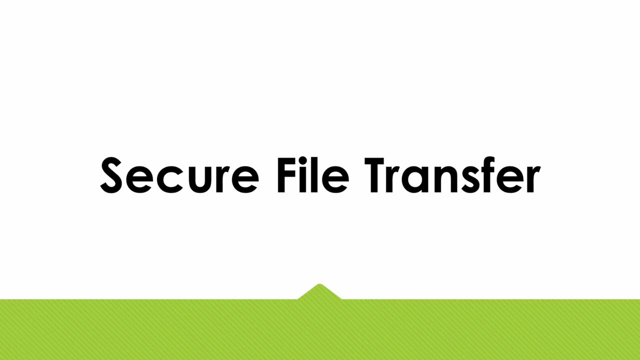 remote location. ssh supports various terminal emulation modes, allowing users to work with different type of terminal environments and shell programs, example bash and zsh. secure file transfer: in addition to terminal access, SSH can be used for secure file transfer between network devices using utilities such as SCP, secure copy protocol and SFTP. that is, SSH file transfer protocol. 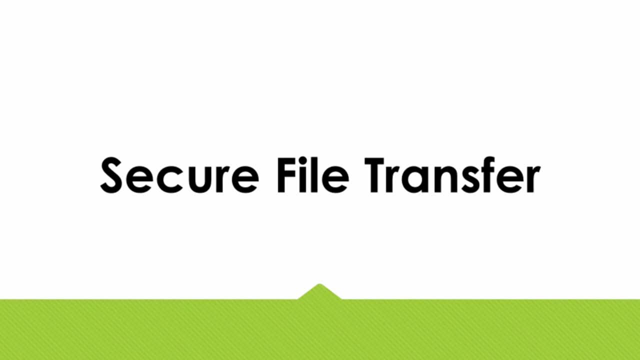 SCP allows users to securely copy files between local and remote systems using the SSH protocol. it provides similar functionalities to the traditional CP command but encrypts data between transmission. SFTP is more advanced protocol that provides a full featured file transfer service over SSH. it supports operations such as file uploads, downloads, directly listing and file. 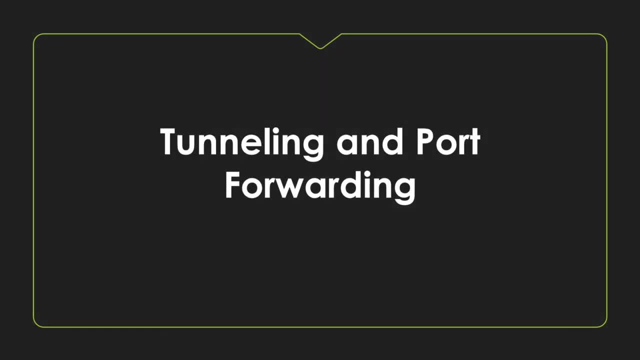 permission management in a secure manner. tunneling and port forwarding: SSH supports tunneling and port forwarding, allowing users to secure and encrypt network traffic between two systems by tunneling it through an SSH connection. SSH can be used for secure file transfer between network devices using utilities. SSH tunneling can be used to secure other network protocols, example HTTP, FTP. 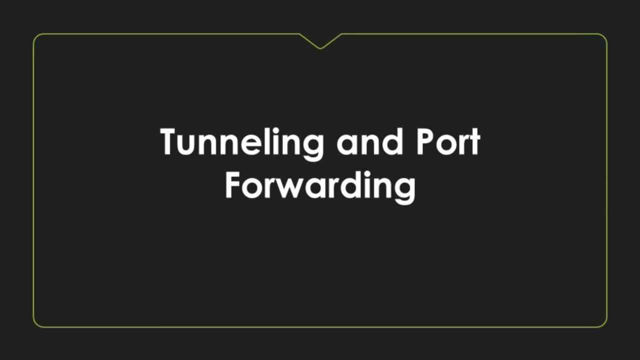 or create encrypted VPN, like connections between systems. port forwarding enables users to forward network traffic from a local port on their system to a remote port on another system via an SSH connection, providing secure access to services running on a remote system. now we will see how you can access a remote. 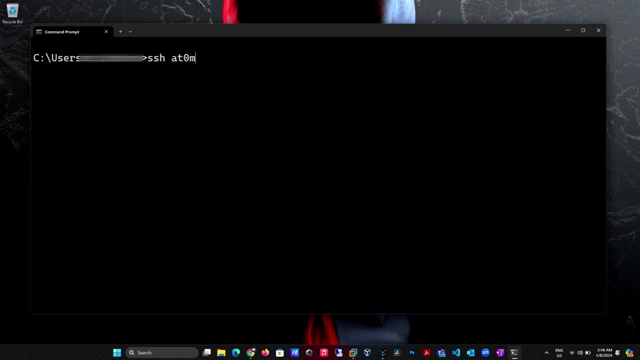 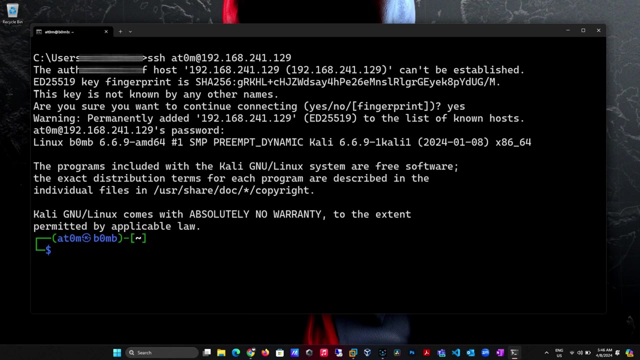 system by using SSH. you will use SSH space username at the rate IP address to access the system. you're going to fingerprint the certificate, so enter yes. after that, write the username password. after authenticating with the correct username and password, you will be presented with the command line interface of the remote 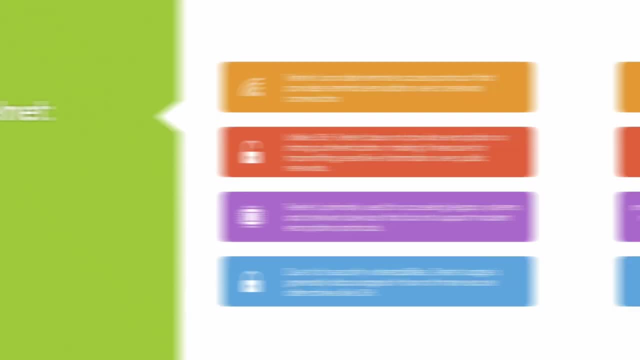 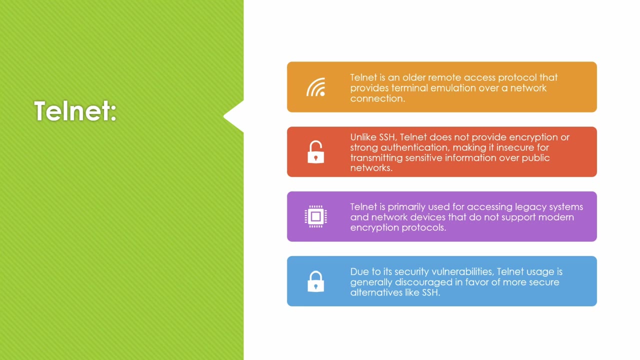 system, and now you can access the system remotely. now we will talk about telnet. telnet is a network protocol used for remote terminal access. it allows a user from one computer to log into another computer that is part of the same network and interact with its command line interface as if they were. 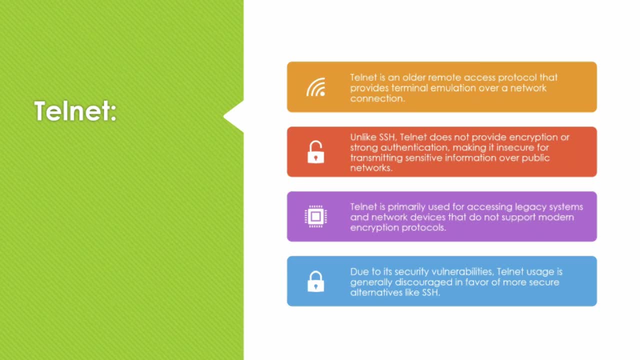 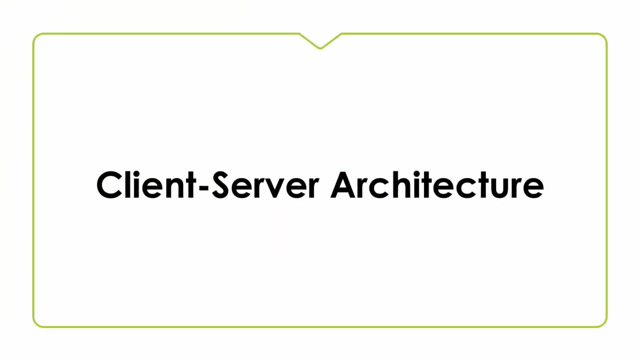 physically present at that remote location. telnet operates over TCP IP networks and provide a simple text-based communication mechanism between client and server system. here's a detailed overview of telnet client server architecture. telnet operates on a client server architecture model, where one system, the telnet client- 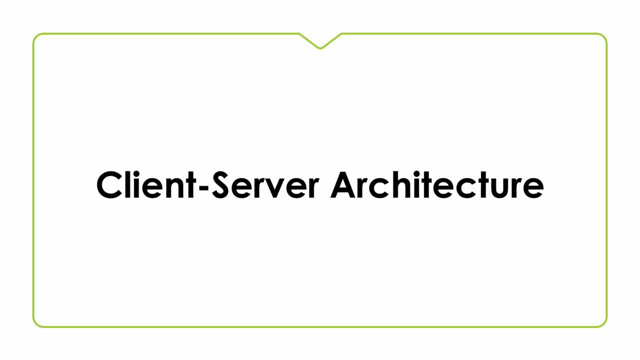 initiates a connection, another system, the telnet server, to establish a remote terminal session. the telnet client software is typically installed on the users local system, allowing them to connect to remote systems and access their command line interface or execute commands remotely. the telnet server software runs on the 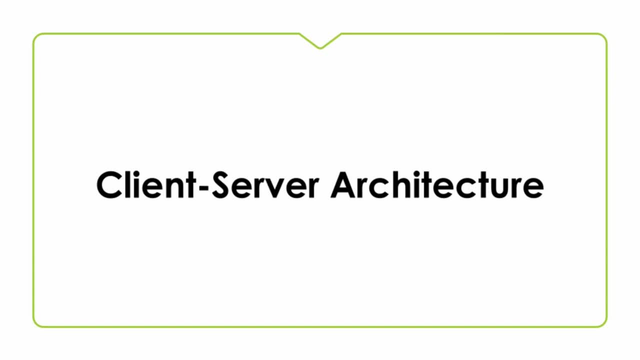 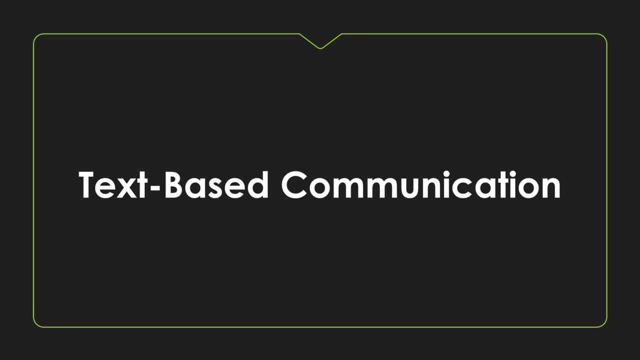 remote system, listening for incoming telnet connections and providing users with access to the command line interface. text-based communication. telnet sessions are text-based, meaning the communication between the client and the server consists of plain text messages exchange over the network. users interact with the remote systems command line interface by 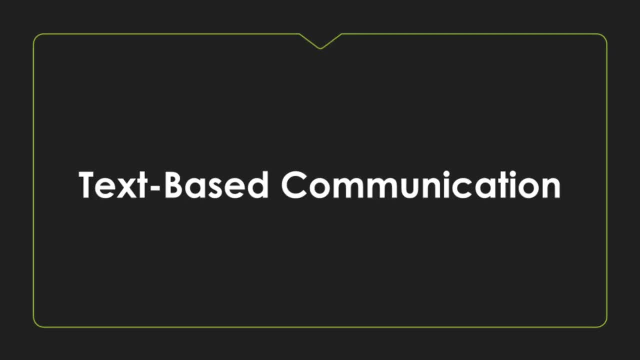 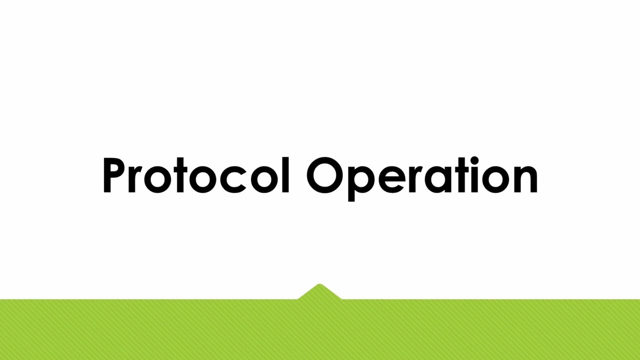 typing commands and receiving text-based responses from the server. telnet does not provide support for graphical user interfaces, GUIs or multimedia content, as it is designed primarily for accessing text based terminals and executing command line operations. protocol operation: telnet uses telnet protocol to felicitate communication between the client and the server through the mobile service and typical 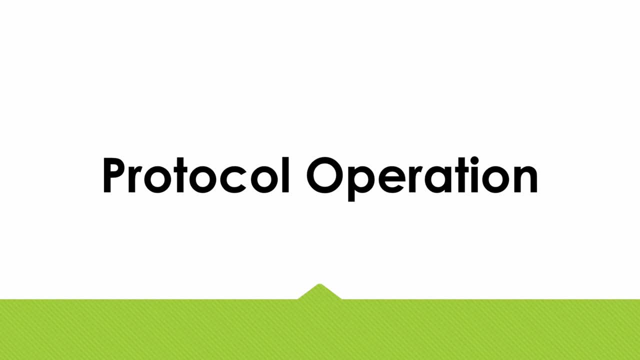 between the client and the server system. The Telnet protocol defines a set of commands and control sequences for negotiating terminal settings, handling inputs and outputs and managing the remote terminal session. Telnet sessions are initialized by establishing a TCP connection between the client and the server system on the default Telnet port, TCP port 23.. 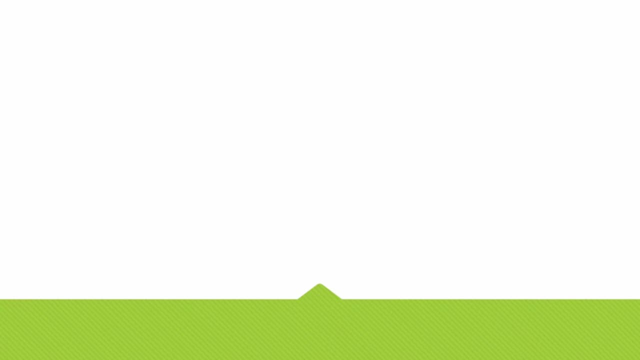 Once the connection is established, the client and server negotiate session parameters and begin the session Security considerations. Telnet session transmits data in plain text, which means that communication between the client and the server is not encrypted. As a result, Telnet is vulnerable. 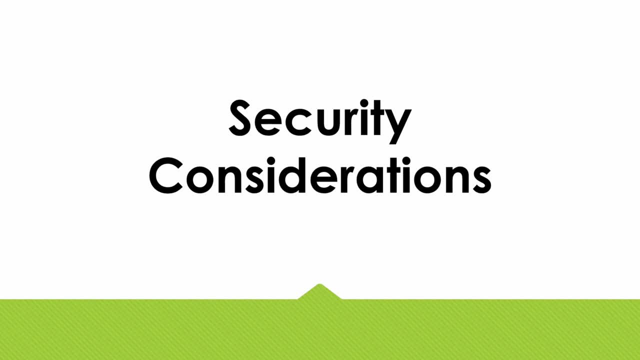 to eavesdropping, packet sniffing and man-in-the-middle attacks, where attackers can intercept and view sensitive information such as login credentials transmitted over the network. Due to its lack of encryption and inherent security risk, Telnet usage is generally discouraged for accessing. 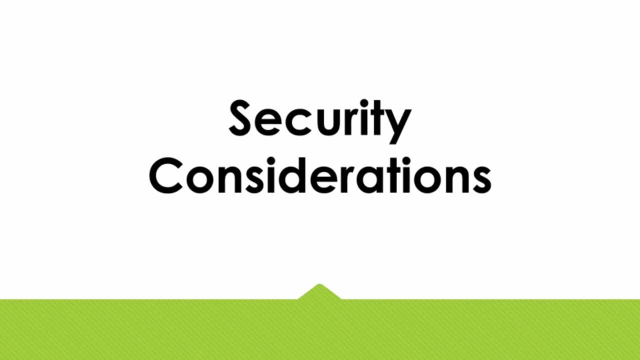 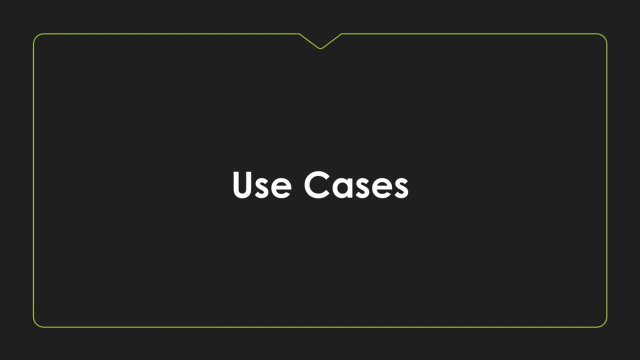 remote sessions systems over untrusted networks, particularly in public internet Use cases. Telnet was historically used for remote administration, troubleshooting and accessing network devices such as servers, routers, switches and printers. It provides a convenient way for system administrators and network engineers to manage and configure remote systems and network. 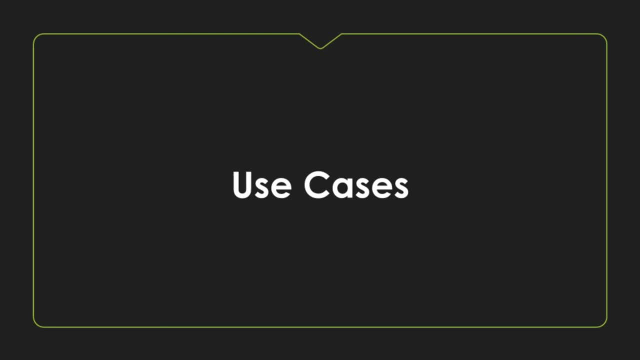 devices without physical access to the equipment. However, due to its security vulnerabilities, Telnet has largely been used as a means of access to the network. Telnet has been replaced by more secure remote access protocols such as SSH, that is, secure shell which offers encryption. 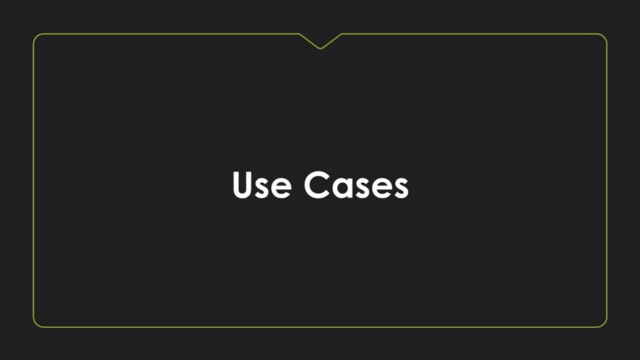 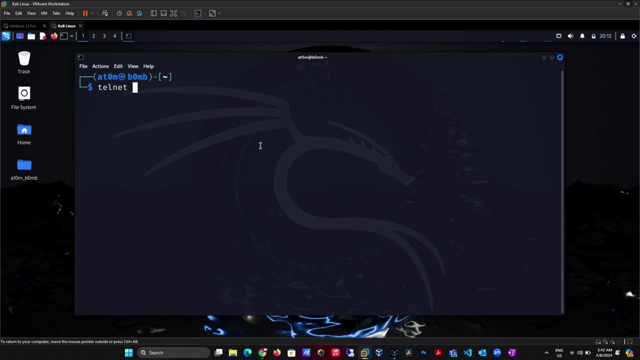 authentication and stronger security features to protect remote communication. All right, now we will see how to remotely connect to a web server that is hosting a web page by using the Telnet protocol. The correct syntax for Telnet is telnet, space, hostname, space, port number. Now we have successfully connected to examplecom.